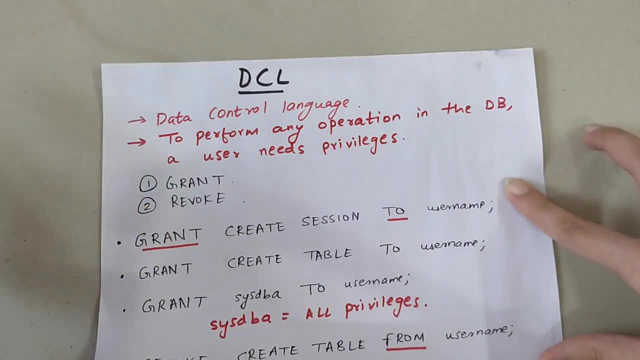 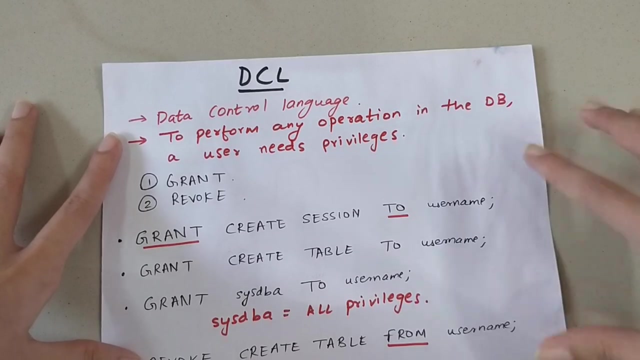 we give a particular permission that this user is allowed to do this, this, this, And the user cannot do this particular operation. So we revoke, we take the permission back which was already given to the user. So let's see some examples of grant and revoke. So first, 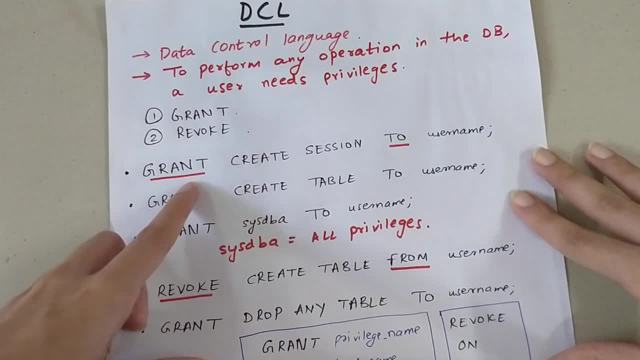 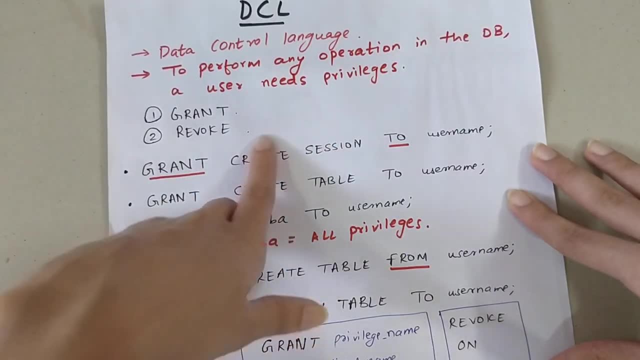 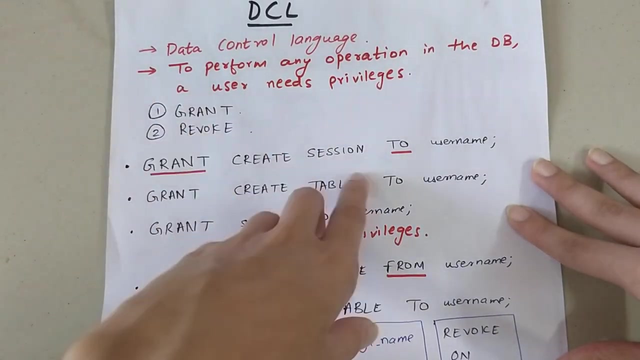 is grant create session to user name. So basically grant means the permission is to be given. What is the operation name- Create session. So basically the user, user name, user can create session and it is given to to what? To user name, So basically to user. 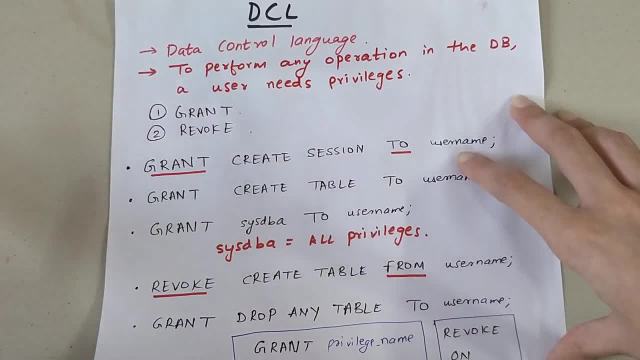 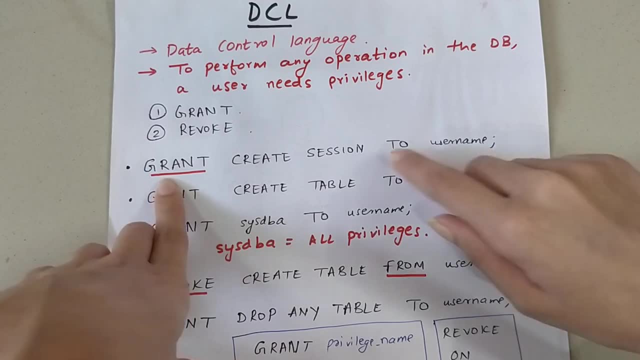 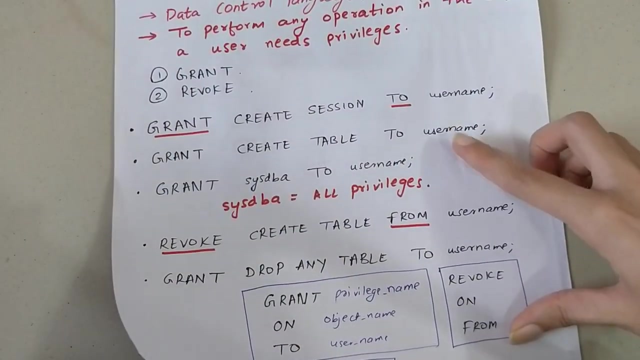 So here the user name of the particular user will be written over here. So user name can be anything. So grant- create session to user name. So in grant we have grant whatever the operation name is this and then to whatever user name. Second is grant- create table to. 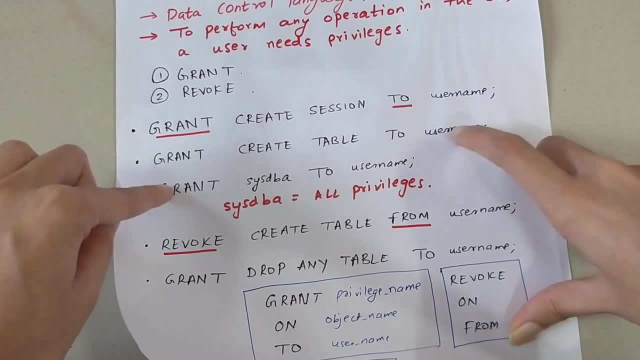 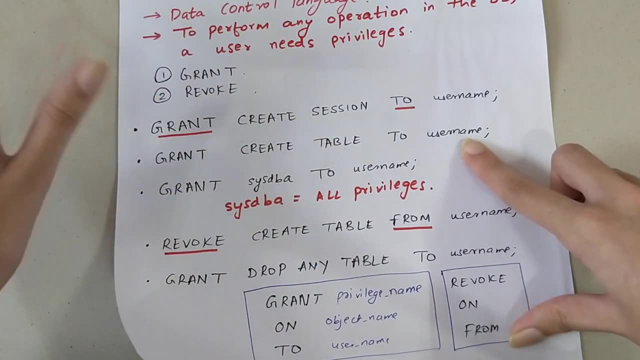 xyz user name, whatever. So basically x is suppose. here we have written xyz, So the xyz user is allowed to create tables in the dba. Okay, So that way we are giving it permission. Third is grant sysdba to user, to user name. Now what? 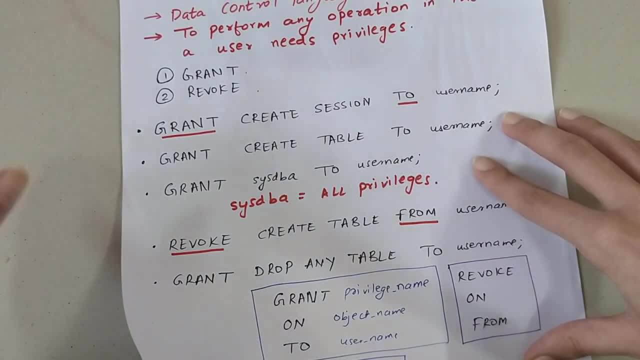 is sysdba. Sysdba means all the privileges. Now you want to give. give a user all the privileges, like that particular user can create, drop, can do anything. So instead of writing one, one operation, we can use the word sysdba. 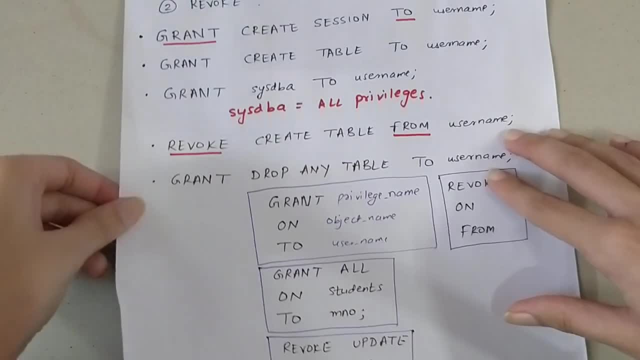 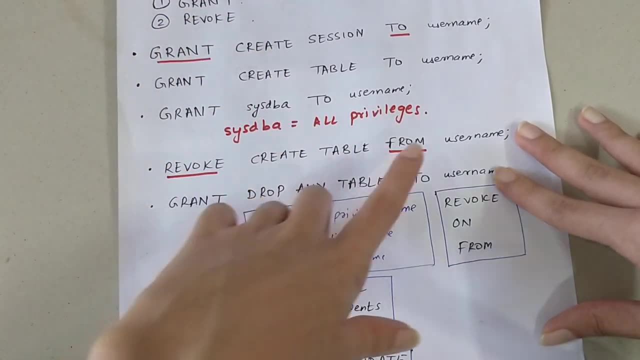 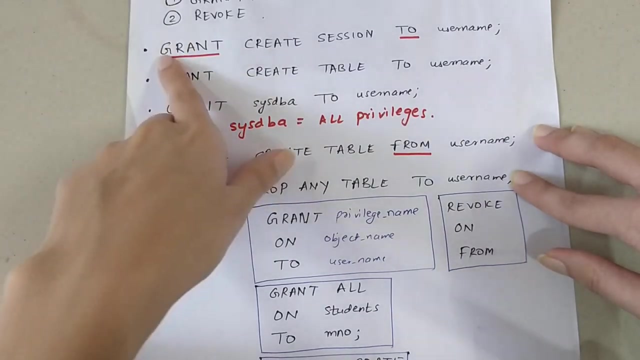 Okay, Now revoke. Now we have to take the permission明公 menus by. still, I forgot. Now we have to take the permission back, the privilege back, So revoke. create table from whichever particular user name. So in case of grant, in case of grant, we have grant. 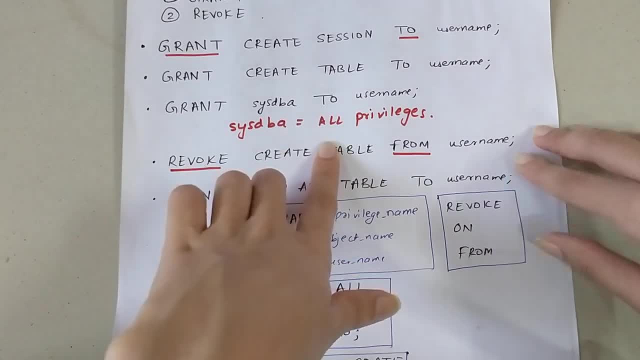 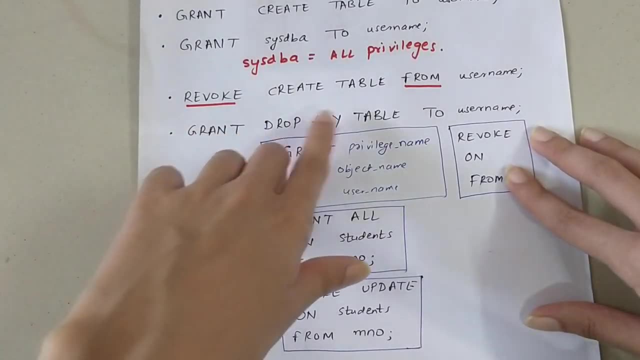 so-and-so to so and so username. Revoke so and so from so-and-so user name. Okay, Now, if you want to grant grant, drop any table now. create the table byantодe creation date DNA, So, and if you want to create or drop any table from any particular table over here the question: